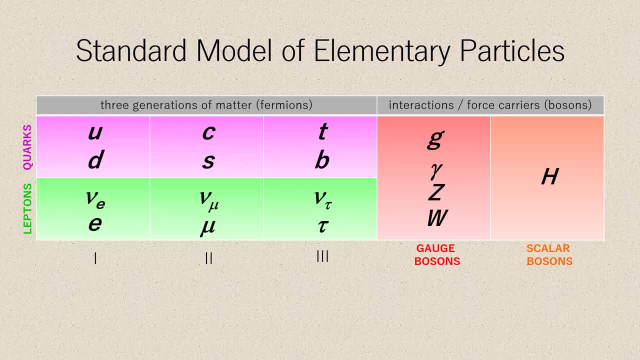 The standard model of particle physics is the theory describing three of the four known fundamental forces- the electromagnetic, weak and strong interactions- and not including the gravitational force in the universe. as well as classifying all known elementary particles, The standard model includes 12 elementary particles of spin 1⁄2, known as fermions. 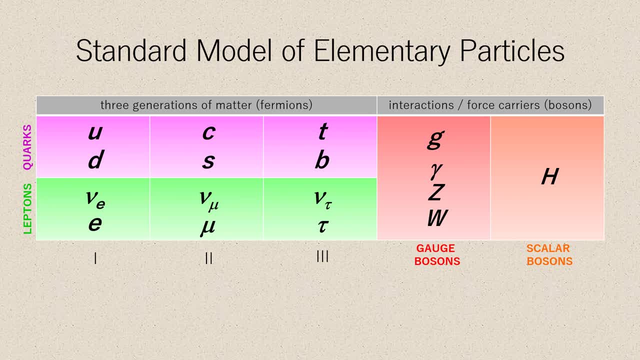 Each fermion has a corresponding antiparticle. The fermions of the standard model are classified according to how they interact. There are six quarks and six lepton's. electron neutron, muon, muon neutron Tau –, TAU neutron. 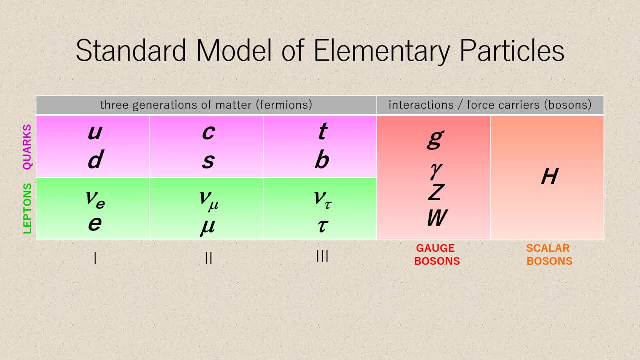 Pairs from each classification are grouped together to form a generation with corresponding particles exhibiting similar physical behavior. The defining property of the quarks is that they carry color charge and hence interact via the strong interaction. Quarks also carry electric charge and weak isospin. 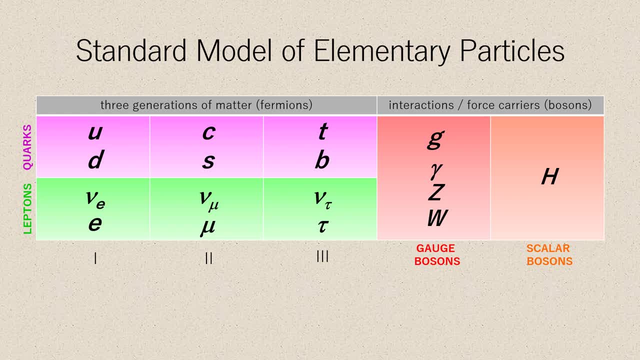 Hence they interact with other fermions both electromagnetically and via the weak interaction. The remaining six fermions do not carry color charge and are called leptons. The three neutrinos do not carry electric charge either, so their motion is directly influenced only by the weak nuclear force. 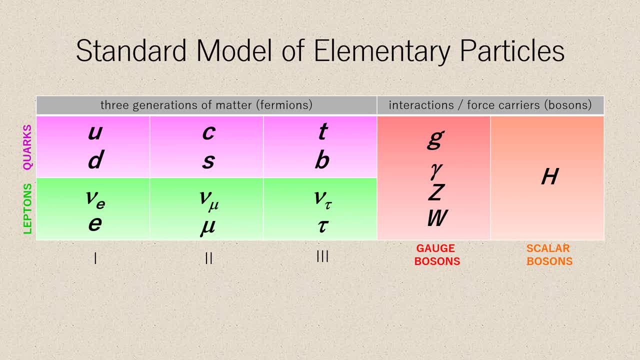 However, by virtue of carrying an electric charge, the electron, muon and tau all interact electromagnetically. Each member of a generation has greater mass than the corresponding particles of lower generations. The first-generation charged particles do not decay, hence all ordinary baryonic matter is made of such particles. 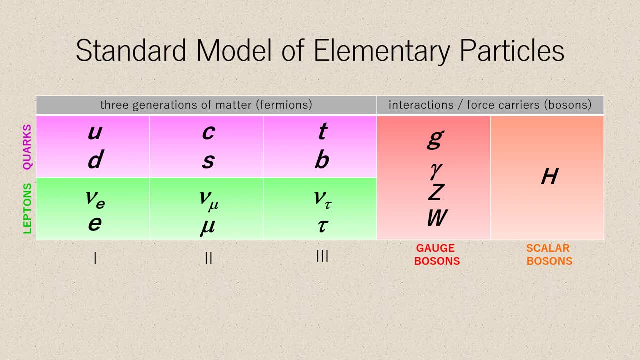 specifically, all atoms consist of electrons orbiting around atomic nuclei, ultimately constituted of up and down quarks. In the standard model gauge, bosons are defined as force carriers that mediate the strong, weak and electromagnetic fundamental interactions. Photons mediate the electromagnetic force between electrically charged particles. 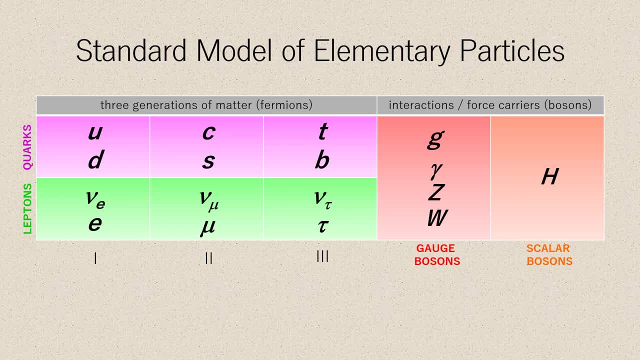 The photon is massless and is well described by the theory of quantum electrodynamics. The W and Z are the same. The Z range bosons mediate the weak interactions between particles of different flavors, all quarks and leptons. They are massive. 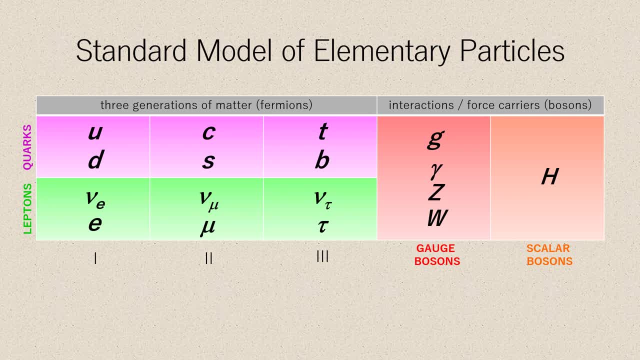 The weak interactions involving the W exclusively act on left-handed particles and right-handed antiparticles. Furthermore, the W carries an electric charge of plus one and minus one and couples to the electromagnetic interaction. The electrically neutral Z boson interacts with both left-handed particles and antiparticles. 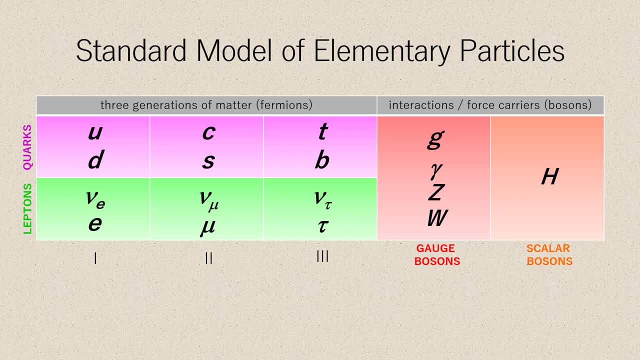 These three gauge bosons, along with the photons, are grouped together as collectively mediating the electroweak interaction. The eight gluons mediate the strong interactions between color-charged particles. the quarks Gluons are massless. The gluons and their interactions are described by the theory of quantum chromodynamics. 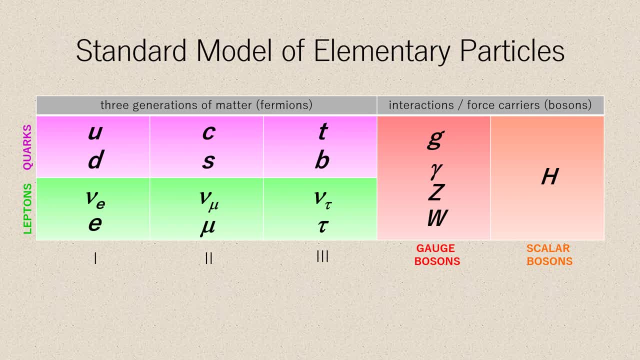 The Higgs particle is a massive scalar elementary particle theorized by Peter Higgs in 1964. It has no intrinsic spin and for that reason is classified as a boson like the gauge bosons, which have integer spin. The Higgs boson plays a unique role in the standard model by explaining why the other 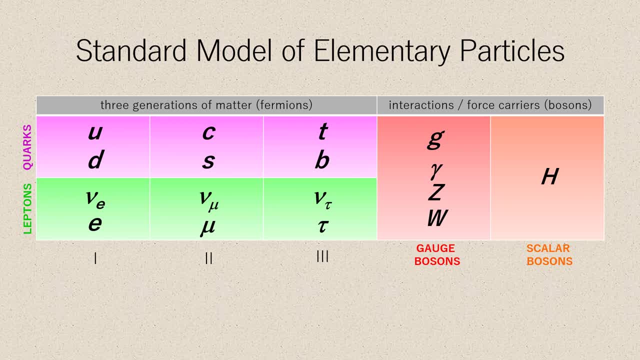 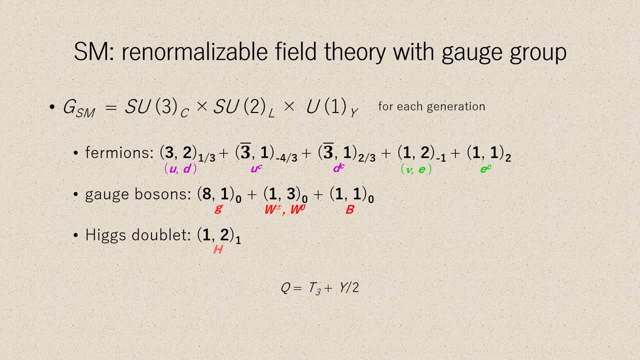 elementary particles, except the photon and gluon, are massive. The standard model may be defined as the renormalizable field theory with gauge group SU3, cross, SU2, cross, U1,, with three generations of fermions in the representation and a scalar Higgs doublet. 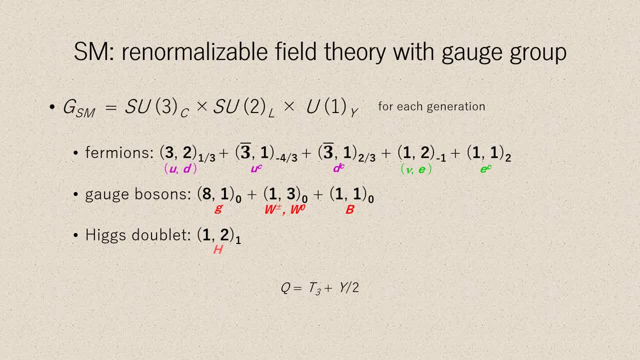 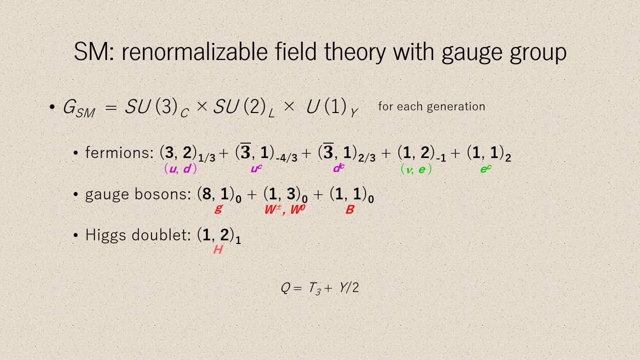 The boldface numbers are the dimension of representations of nonabelian groups and lower indices for U1 charges. The matter fields should also be familiar as up down, anti-up, anti-down, electron-neutrino electron and anti-electron, called positron for the first generation, with up and down. 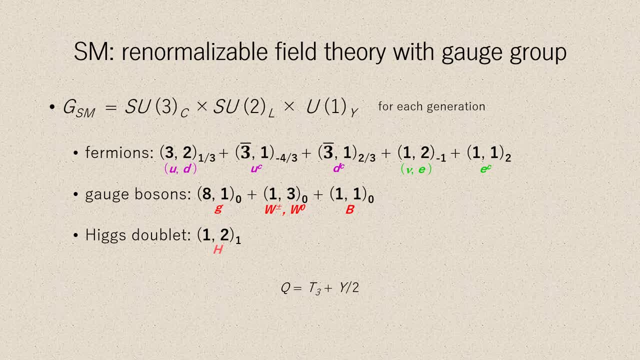 and neutrino and electron being the quark and lepton SU2 doublets and anti-up, anti-down positron as charge conjugate SU2 singlets. The 12 adjoint gauge fields decompose under SU3 cross, SU2 cross- U1.. 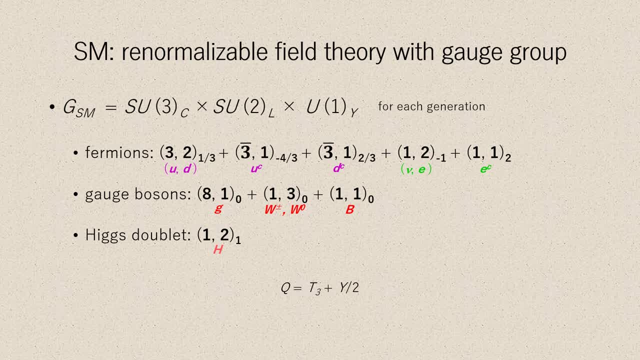 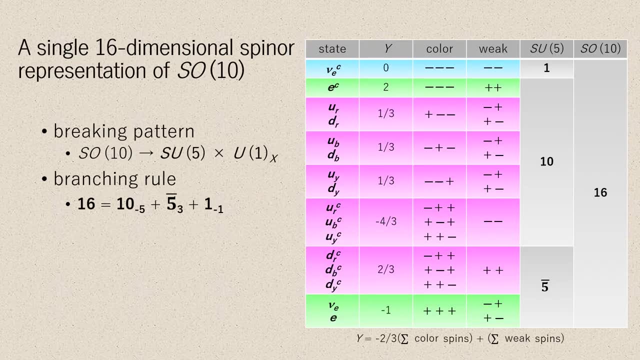 Especially after the recent discovery of the Higgs in 2012,. this model is remarkably complete and consistent with almost all experimental data. A single 16-dimensional spinor representation of SO10 accommodates a full standard model generation together with an extra singlet, potentially providing a right-handed neutrino. 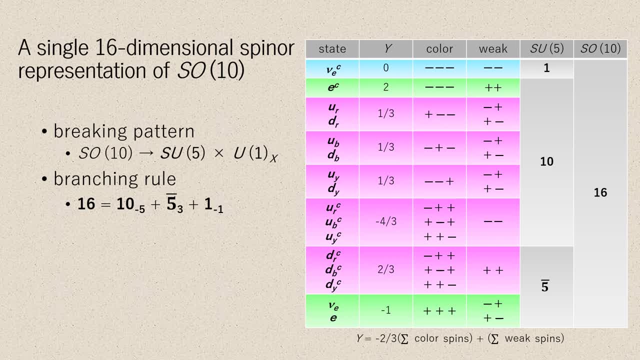 This is most easily understood from the breaking pattern. SO10 goes to SU5, cross U1X and the associated branching rule. Here the indices refer to charges under the U1X subgroup. The table presents the states of one family of quarks and leptons as they appear in the 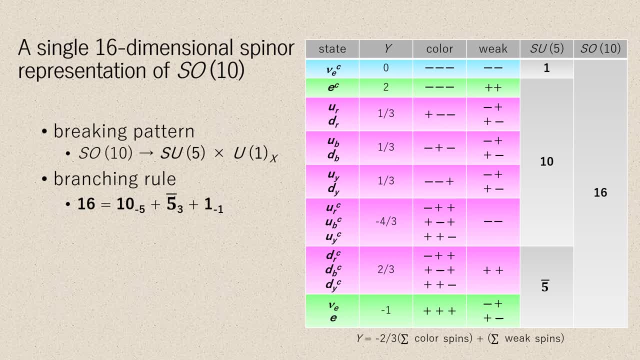 16. The first three and last two spins correspond to SU3 and SU2, respectively. An SU3 rotation just raises one color index and lowers another. The index is written in the form of a quark. Su2 supra changes its orientation to the second spin with two approximate uncertainty. 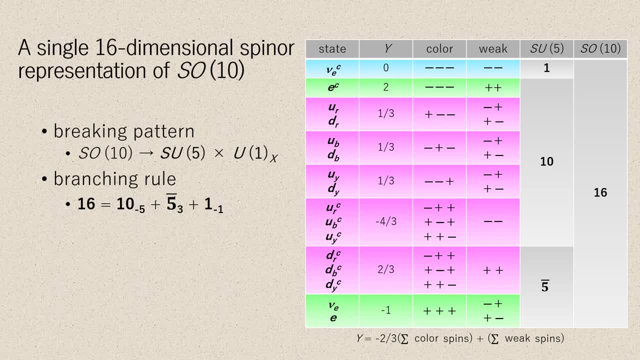 expressions раз side Physics and by Shang and Yang terms used in the process of correlation. Secondly, SU2 change the rotation mechanism into a felicitation function between two spines. Get this example also within SU2.. And if the spin runs at has been used before, which is the result of a quark rotation, then 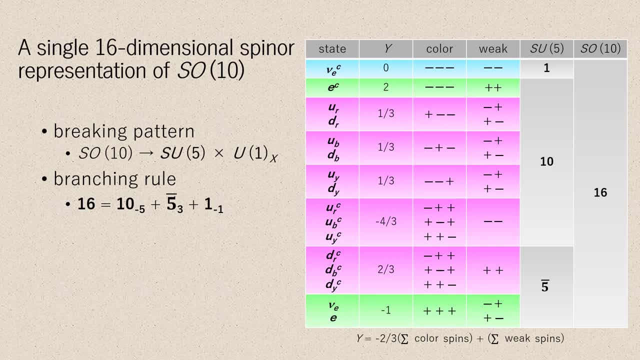 both levitation equations can be applied. Think about this concept for alguma sheets and對啊. So what did we learn? based on this simplification, Such rotations can mix the states up down anti-up positron and anti-down neutrino electron among themselves, and antineutrino is a singlet. 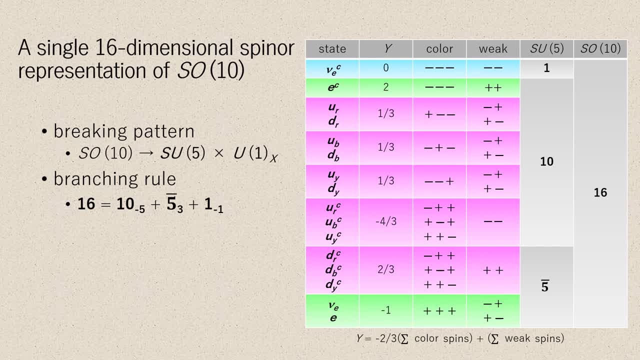 Grand unification means that the standard model gauge interactions of U1, SU2 and SU3 become part of a larger unifying gauge symmetry at a high energy scale. In most models, especially in the simplest and most appealing variants of SU5 and SO10 unification, one expects the three gauge couplings to unify at a unique scale and the proton to be unstable due to exchange of gauge bosons of the larger symmetry group. 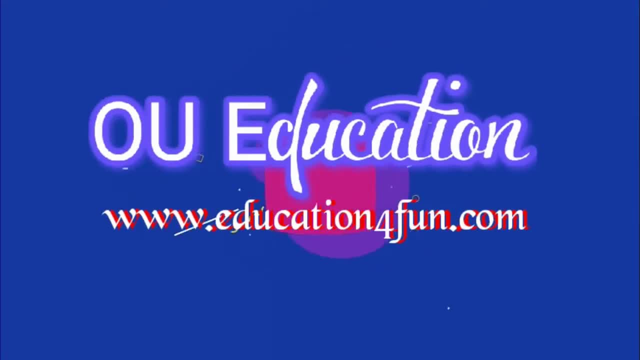 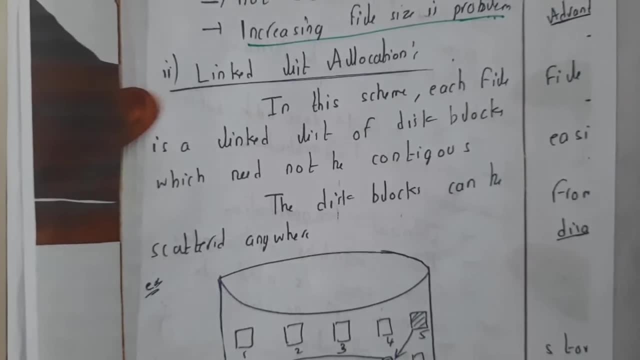 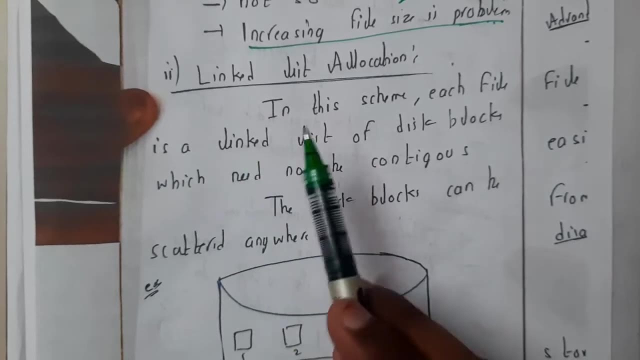 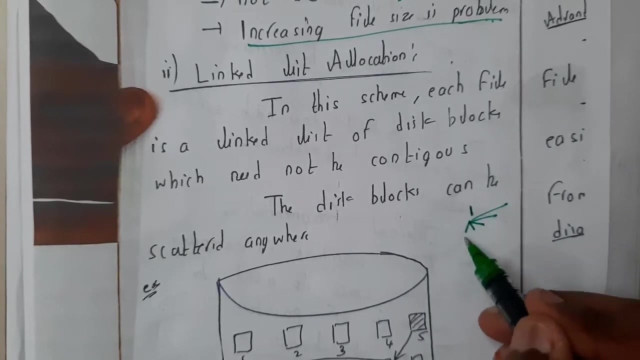 Hello guys, we are back with our next tutorial. In this tutorial let us go through linked list allocation. In this scheme, each file is a linked list, So basically each file will be divided into linked list. So let us assume there is a single file which is divided into five parts, So each